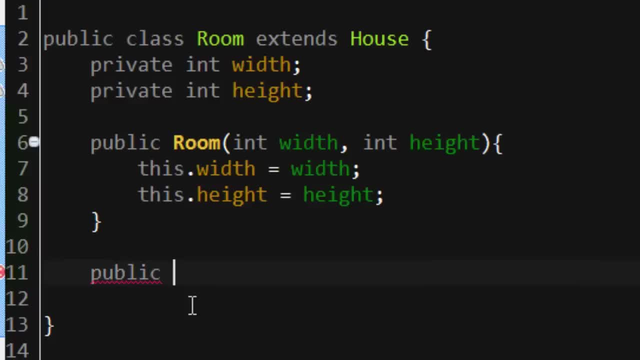 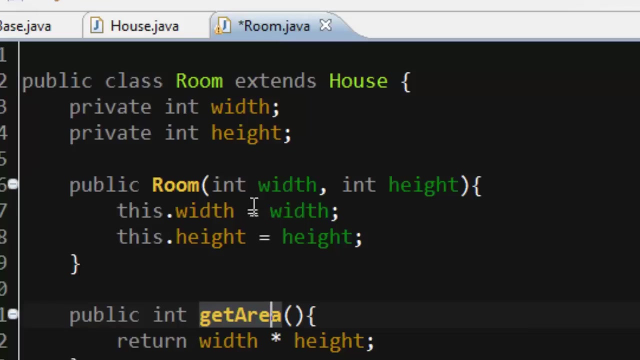 have to do that. So I'm going to declare another function, though called public void, public int get area, and then this get area actually returns width times height, And so we just say that if you want to get an area, let's get. you know something like that. Now we 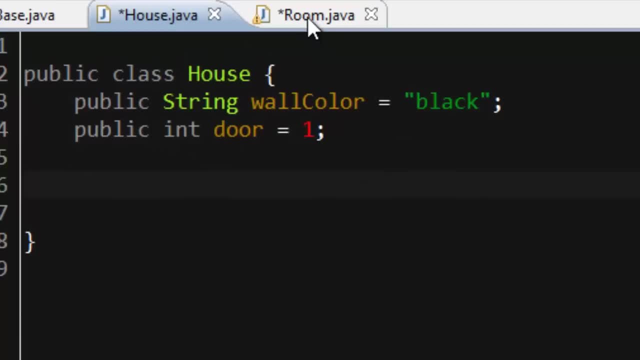 are now going to deal with inheritance. When we say room extends house, we are saying that the room will get everything that is not private though, So it will get everything from house that is not private. Okay, So we just have properties here or members defined here, called. 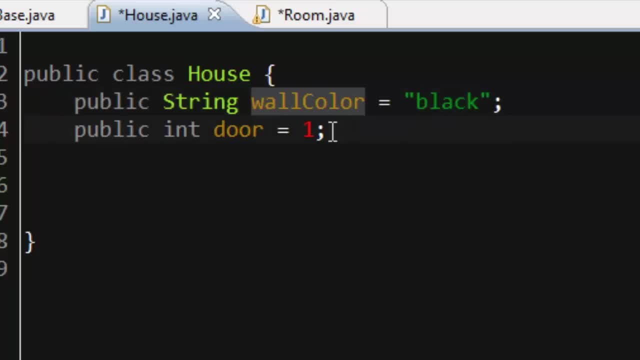 wallpaper or word color and door. But I'm going to define other properties like a method called public void. cool, If you want to cool the house, you have something like public system without the println And the house, the room, cool the house. So I'm going to define a system. 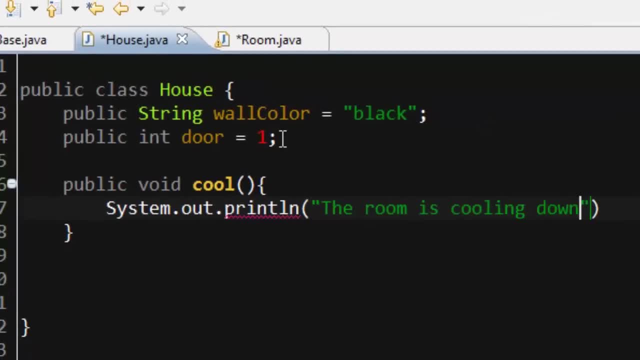 called public void. So I'm going to define a system called public void. So I'm going to define a system called alliiej pray, warm, déjardin, Okay. And then another method here called public cool, warm, And this method says communicate with API And it says the room is warm enough. 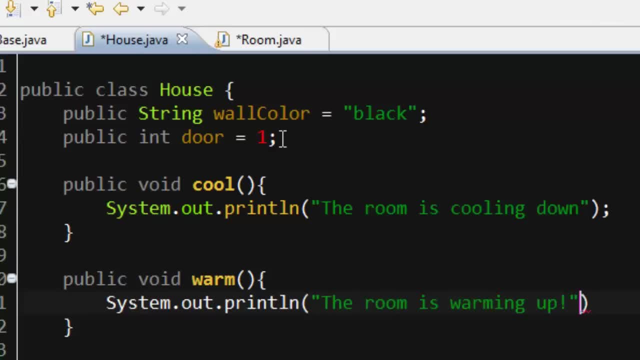 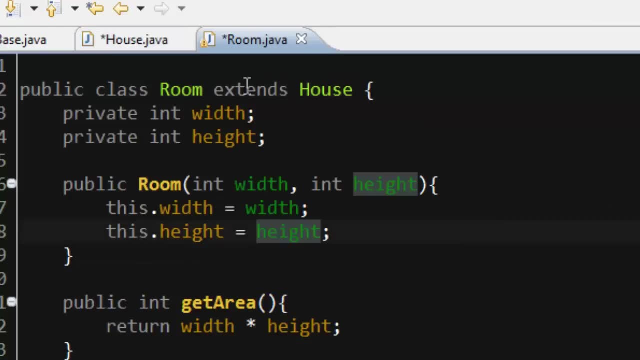 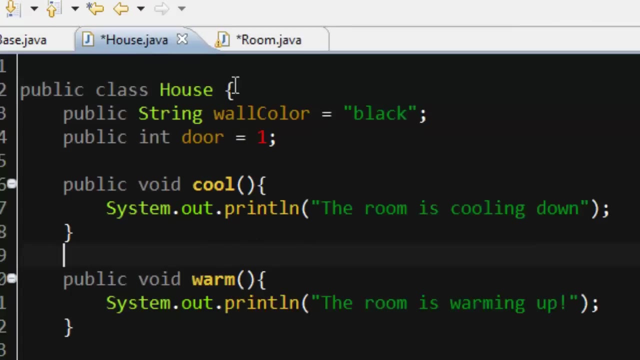 Simple, Right. So, as you can see, we don't have these methods inside the room as we do right now, because it inherits from the house. so the room inherits the cooling and the warming effect from the house. so we can now go ahead and call. you know, call. 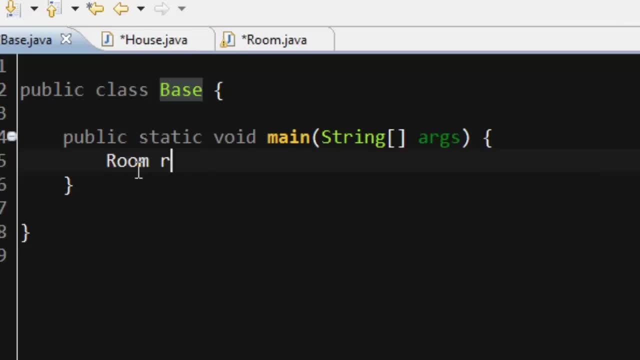 those methods. but first we have to create a room. so let's say room room one was new room and then we pass in something like 12 by 40 in and we have a room called room one. we can now say room one, dot. cool, okay if we say room one.